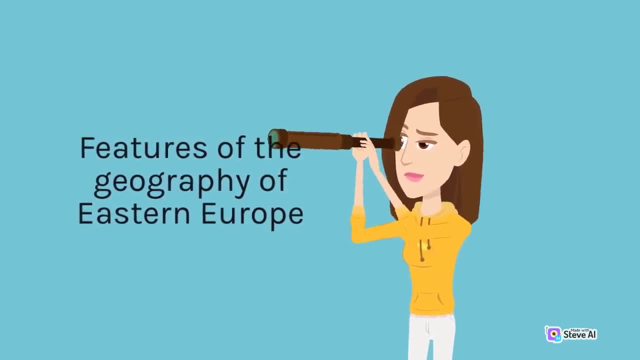 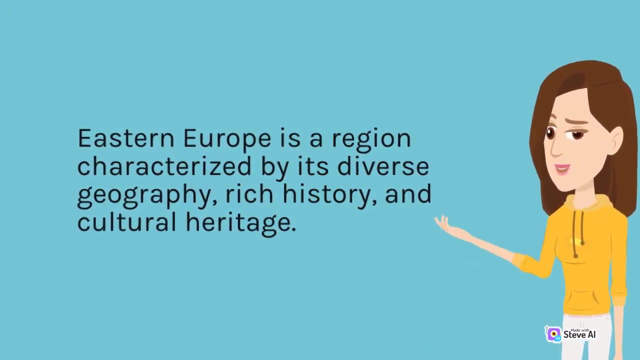 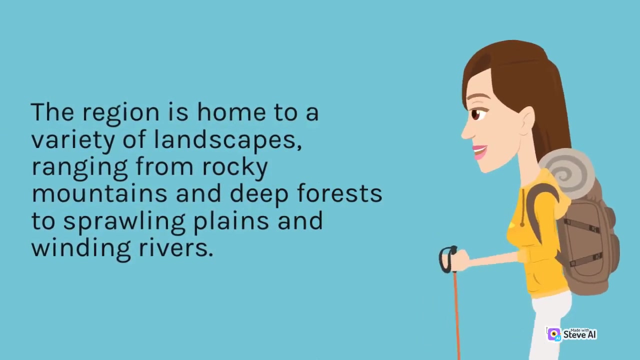 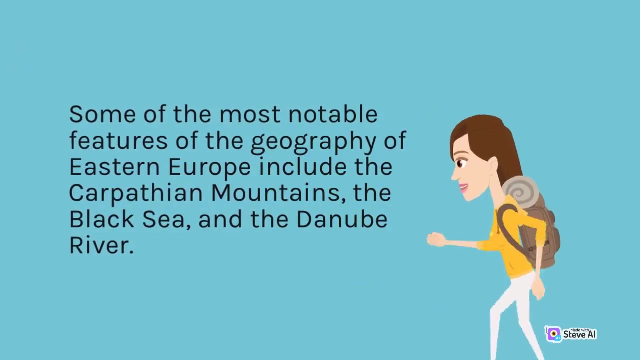 Features of the Geography of Eastern Europe. Eastern Europe is a region characterized by its diverse geography, rich history and cultural heritage. The region is home to a variety of landscapes, ranging from rocky mountains and deep forests to sprawling plains and winding rivers. Some of the most notable features of the geography of Eastern Europe include the Carpathian Mountains, the Black Sea and the Danube River. 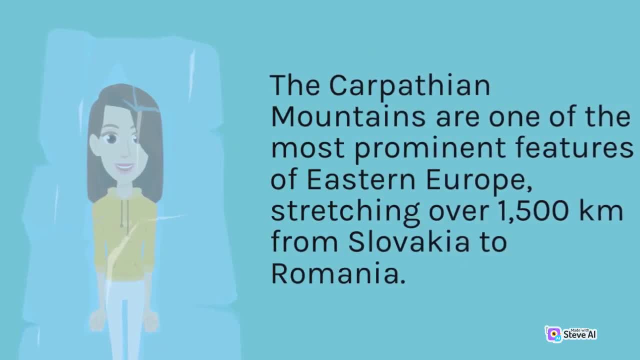 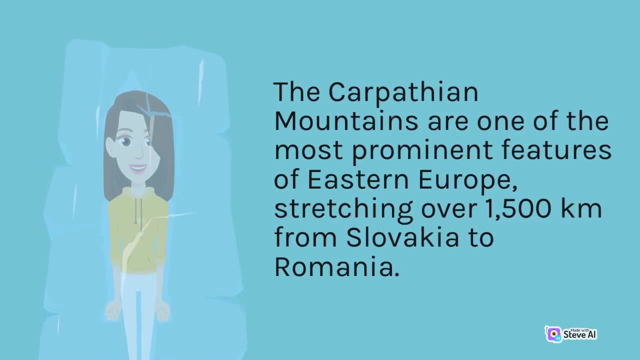 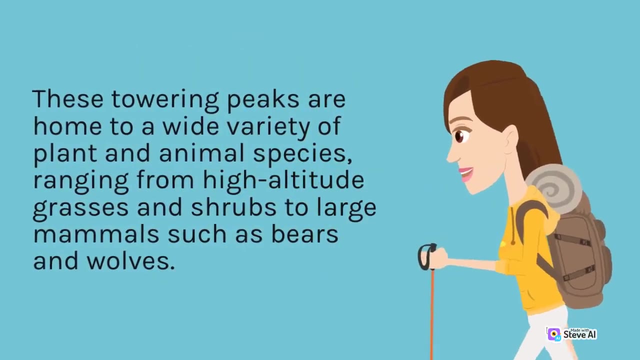 The Carpathian Mountains are one of the most prominent features of Eastern Europe. stretching over 1,500 kilometers from Slovakia to Romania, These towering peaks are home to a wide variety of plant and animal species, ranging from high-altitude grasses and shrubs to large mammals such as bears and wolves. 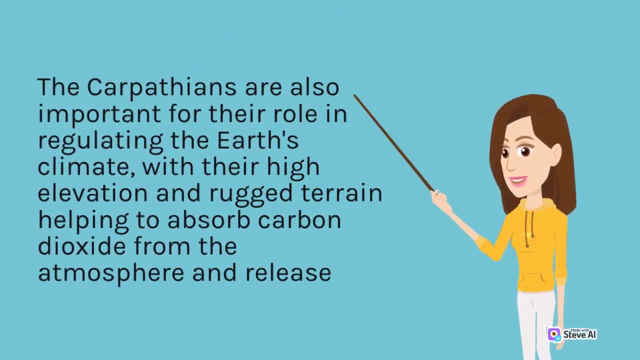 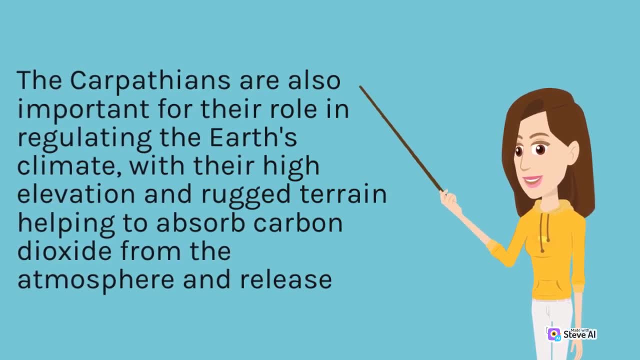 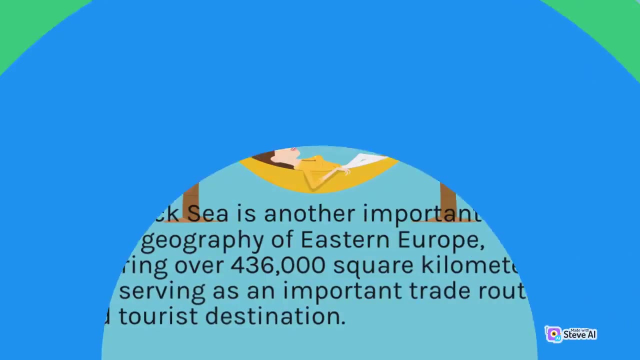 The Carpathians are also important for their role in regulating the Earth's climate, with their high elevation and high climate. The Carpathians are also important for their role in regulating the Earth's climate, with their high elevation and high climate. The Carpathians are also important for their role in regulating the Earth's climate, with their high elevation and high climate. 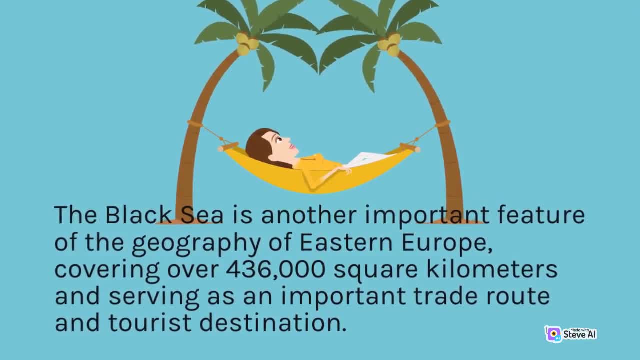 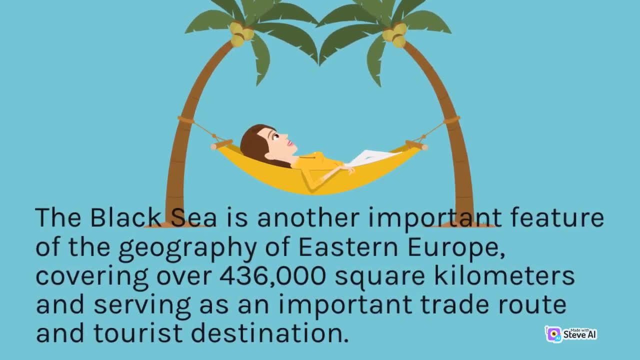 The black sea is another important feature of the Geography of Eastern Europe, covering over 436,000 square kilometers and serving as an important trade route and tourist destination. The Black Sea is home to a wide variety of plant and animal species, including dolphins, seals and a variety of species. 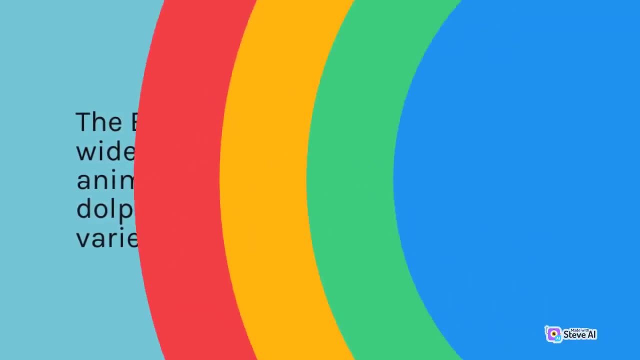 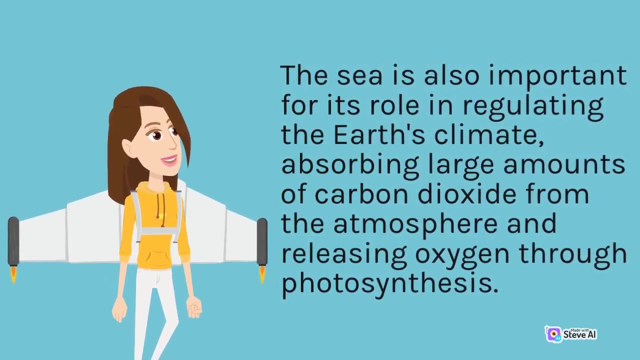 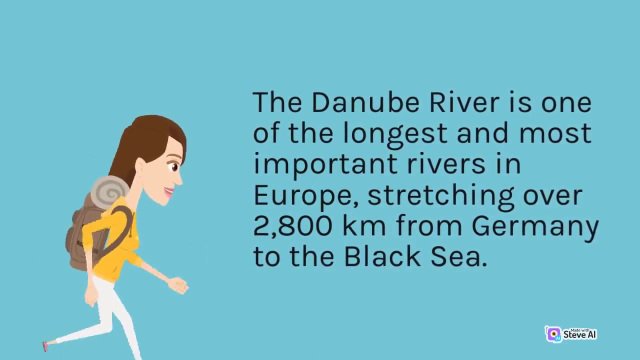 variety of fish species. The sea is also important for its role in regulating the Earth's climate, absorbing large amounts of carbon dioxide from the atmosphere and releasing oxygen through photosynthesis. The Danube River is one of the longest and most important rivers in Europe, stretching 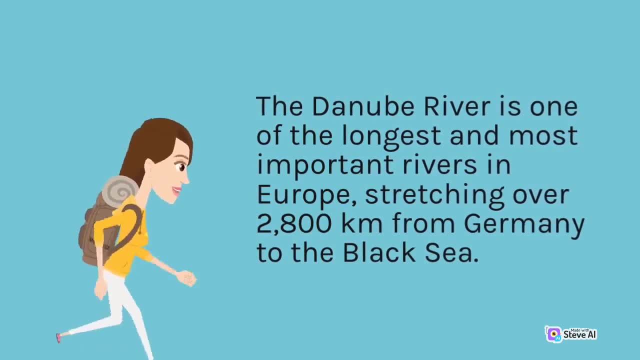 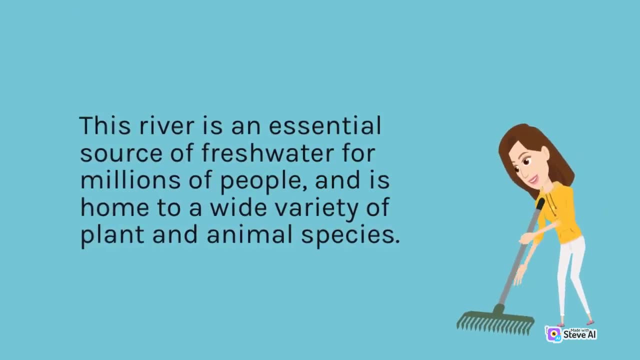 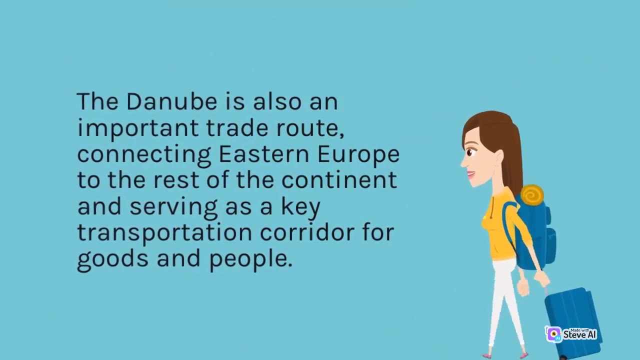 over 2,800 kilometers from Germany to the Black Sea. This river is an essential source of fresh water for millions of people and is home to a wide variety of plant and animal species. The Danube is also an important trade route connecting Eastern Europe to the rest of the 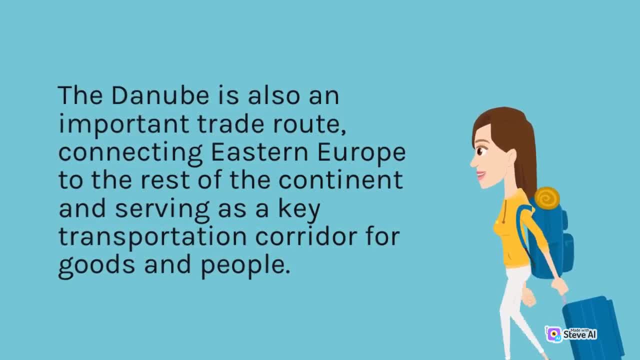 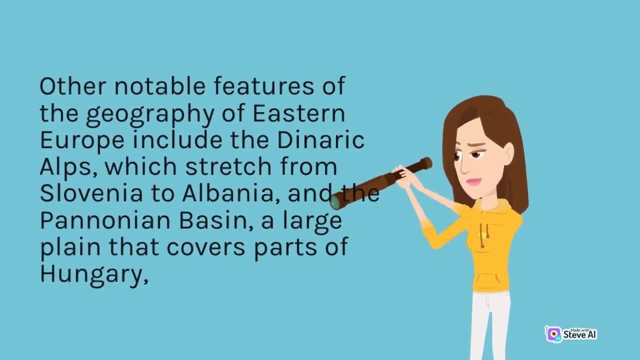 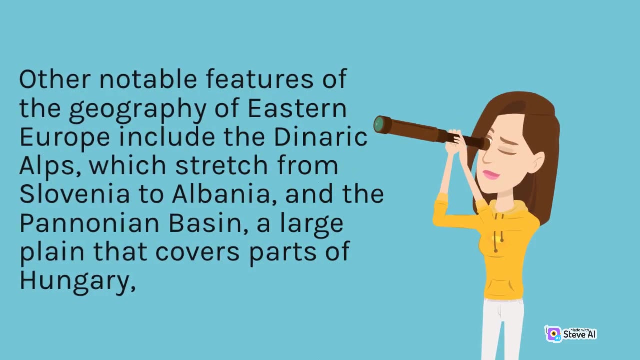 continent and serving as a key transportation corridor for goods and people. Other notable features of the geography of Eastern Europe include the Danaric Alps, which stretch from Slovenia to Albania, and the Pannonian Basin, a large plain that covers parts of Hungary. 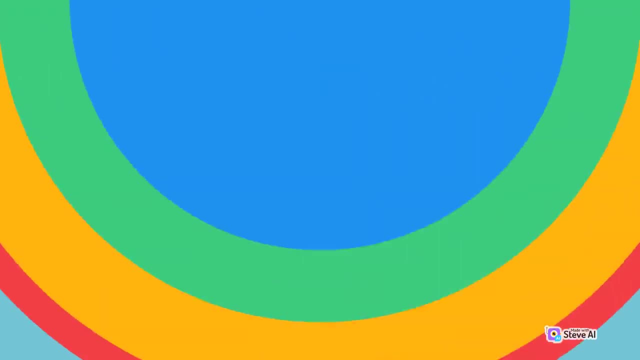 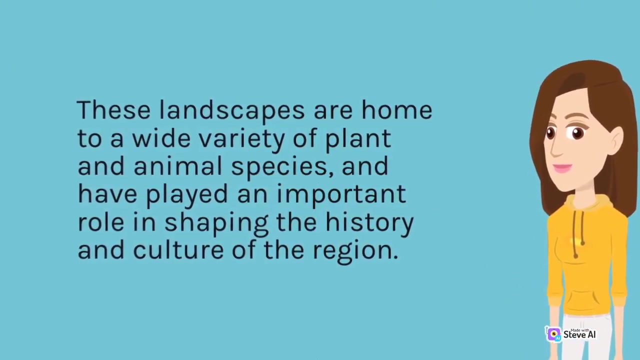 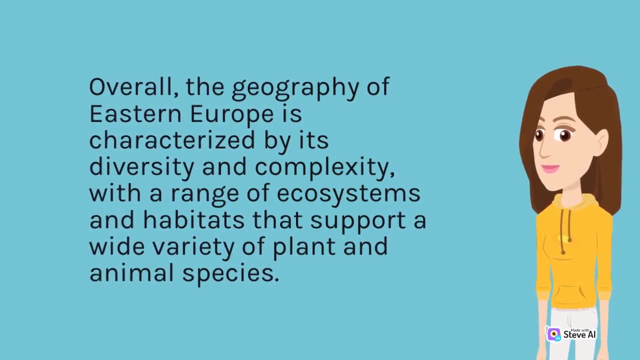 Serbia and Croatia. These landscapes are home to a wide variety of plant and animal species and have played an important role in shaping the history and culture of the region. Overall, the geography of Eastern Europe is characterized by its diversity and complexity, with a range of ecosystems and habitats that support a wide variety of plant and animal. 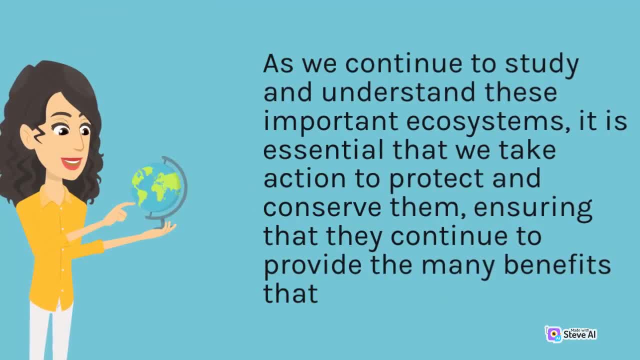 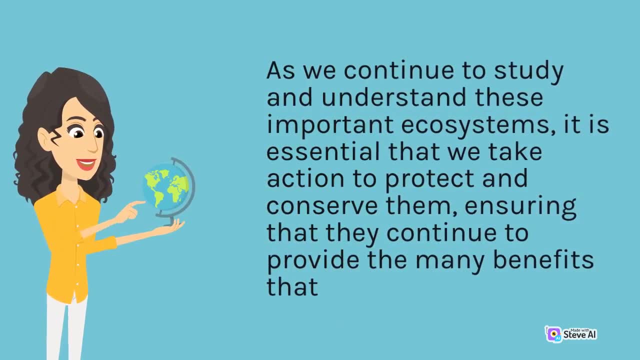 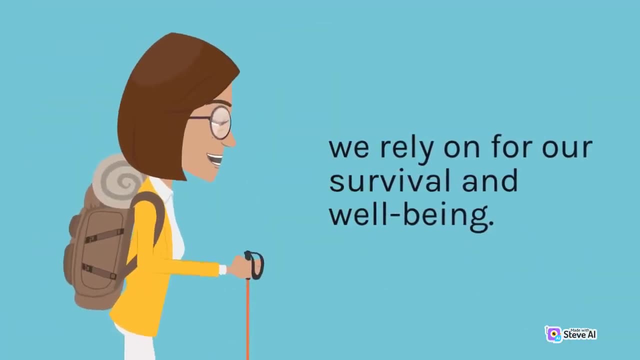 species. As we continue to study and understand these important ecosystems, it is essential that we take action to protect and conserve them, ensuring that they continue to provide the many benefits that we rely on for our survival and well-being. Eastern Europe refers to the region lying culturally and geographically between Western 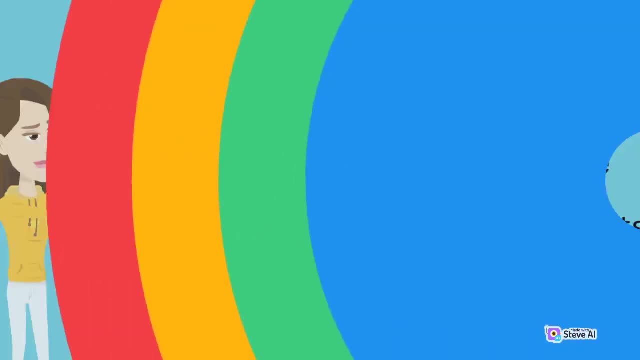 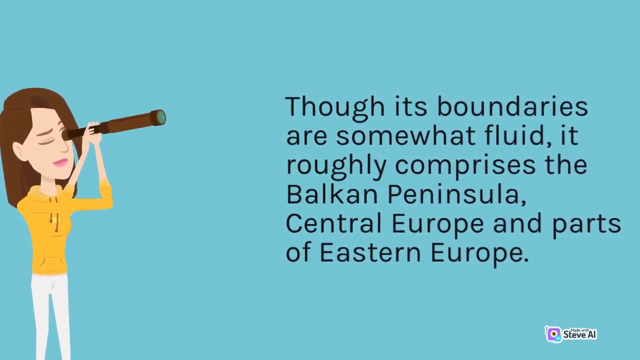 Europe and Asia. Though its boundaries are somewhat fluid, it roughly comprises the Balkan Peninsula, Central Europe and parts of Eastern Europe. The Danube is the largest and most populous continent in the world. The Danube is the largest and most populous continent in the world. 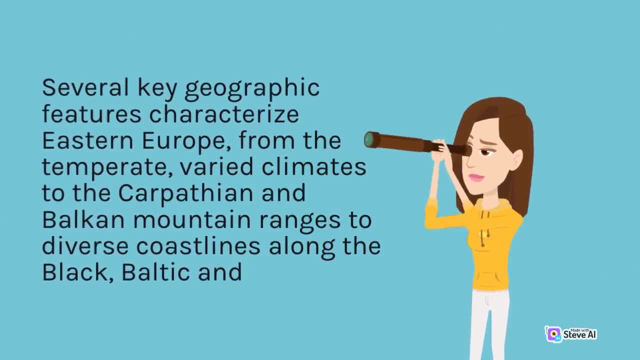 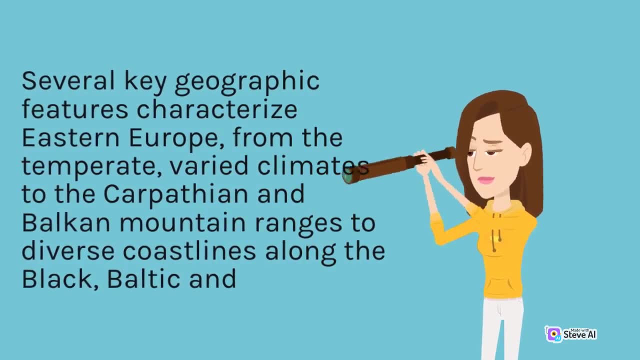 The Danube is the largest and most populous continent in the world. Its geographical features characterize Eastern Europe, from the temperate, varied climates to the Carpathian and Balkan mountain ranges, to diverse coastlines along the Black, Baltic and Aegean seas. 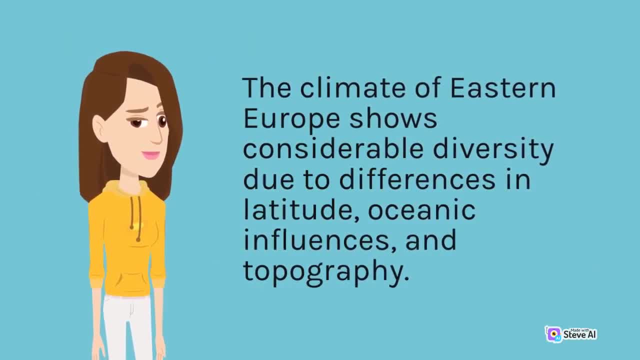 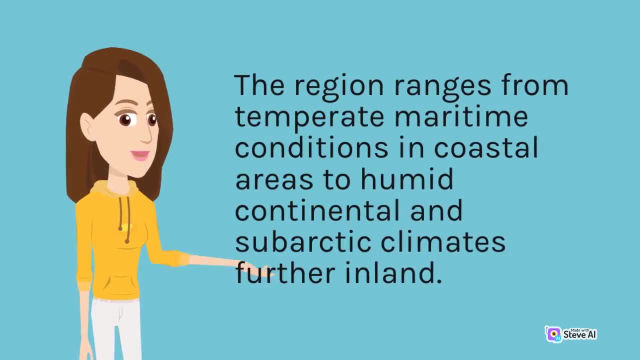 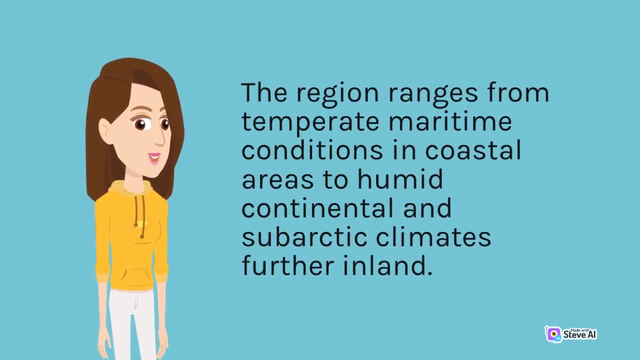 The climate of Eastern Europe shows considerable diversity due to differences in latitude, oceanic influences and topography. The region ranges from temperate maritime conditions in coastal areas to humid continental and subarctic climates. further inland Summers tend to be warm and sunny in most areas, while 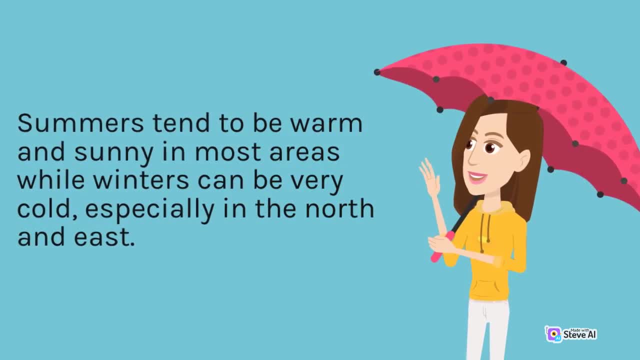 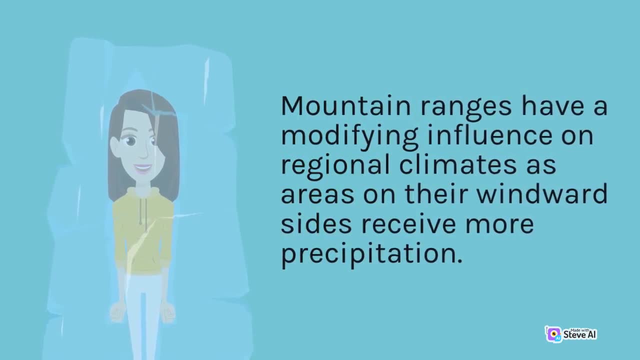 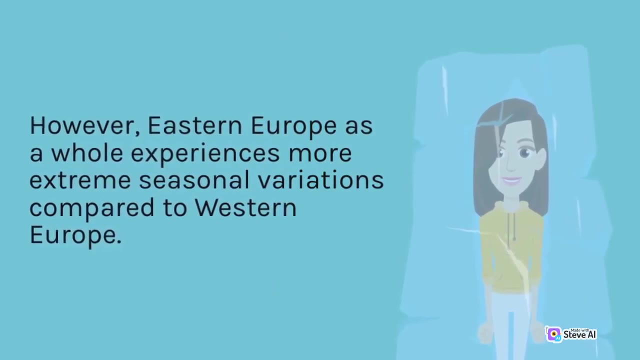 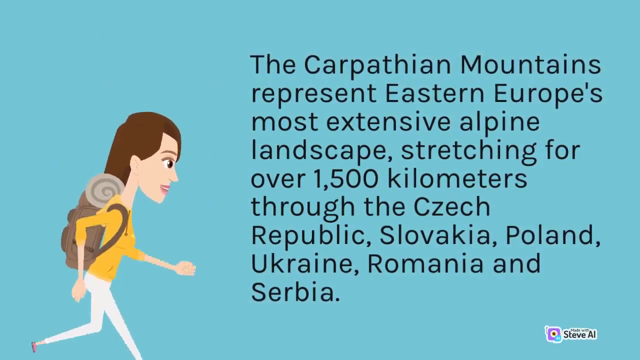 winters can be very cold, especially in the north and east Mound, and ranges have a modifying influence on regional climates as areas on their windward sides receive more precipitation. However, Eastern Europe as a whole experiences more extreme seasonal variations compared to Western Europe. The Carpathian Mountains represent Eastern Europe's most extensive 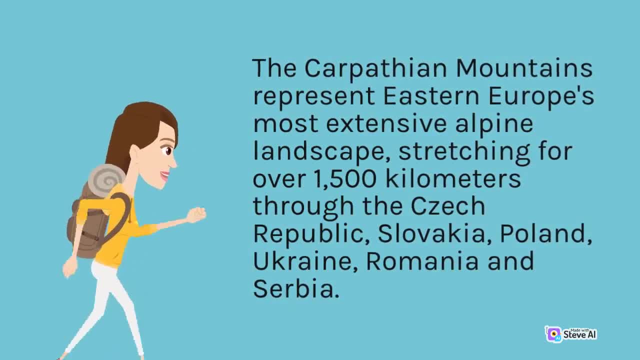 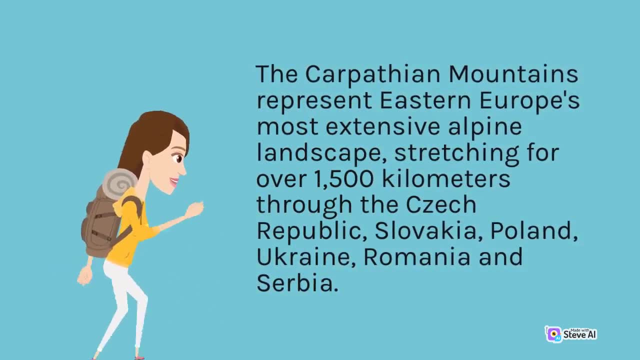 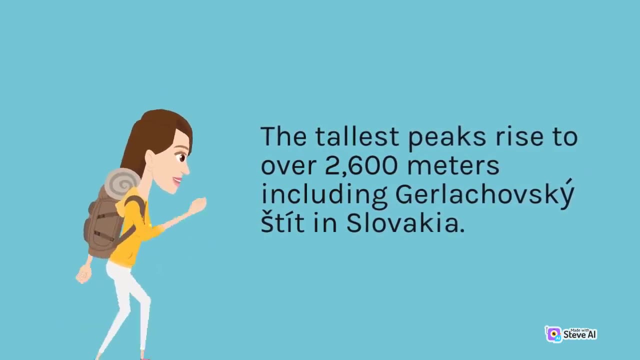 alpine landscape stretching for over 1,500 kilometers through the Czech Republic, Slovakia, Poland, Ukraine, Romania and Serbia. The tallest peaks rise to over 2,600 meters, including Jelajkowski Stid in Slovakia. The Carpathian support diverse vegetation types ranging from